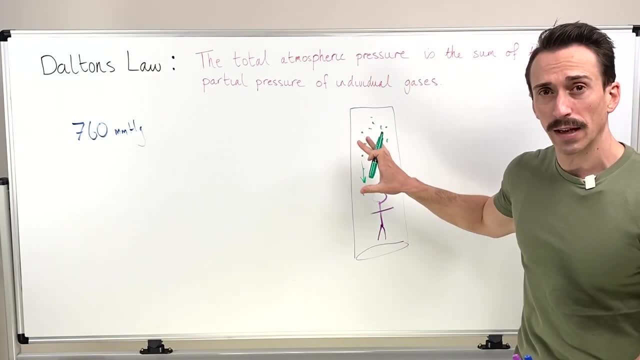 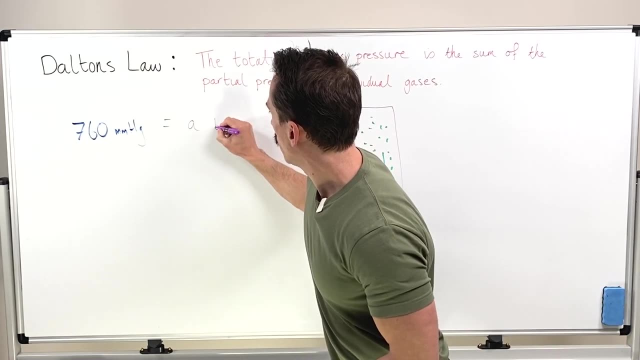 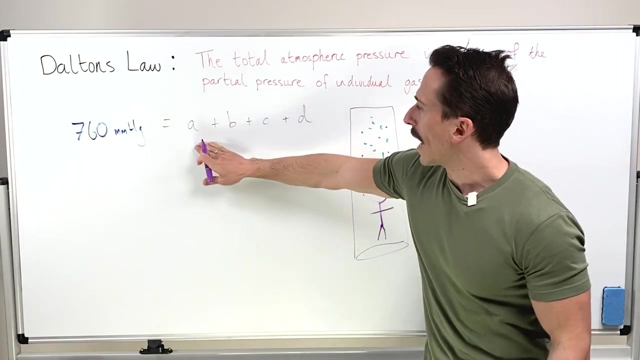 take all the individual gases that make up the atmosphere and add them together. So, for example, 760 millimeters of mercury is equal to A plus B, plus C plus D, for example. So we just need to know what's A, what's B, what's C, what's D. Let's take a look So. 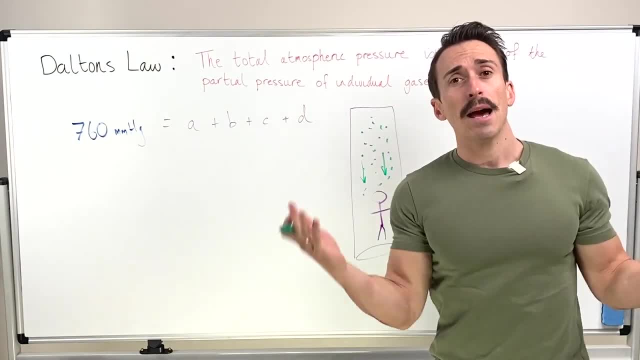 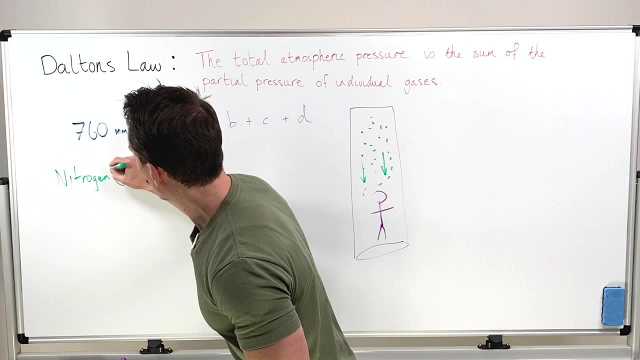 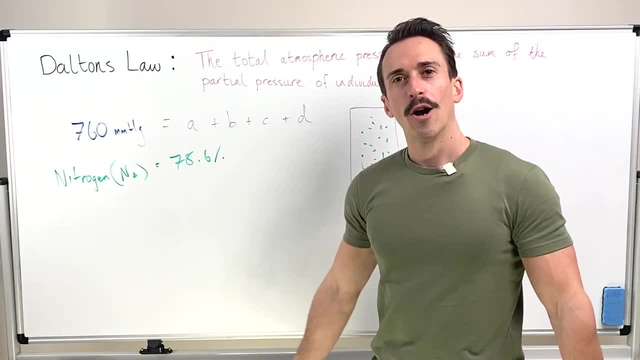 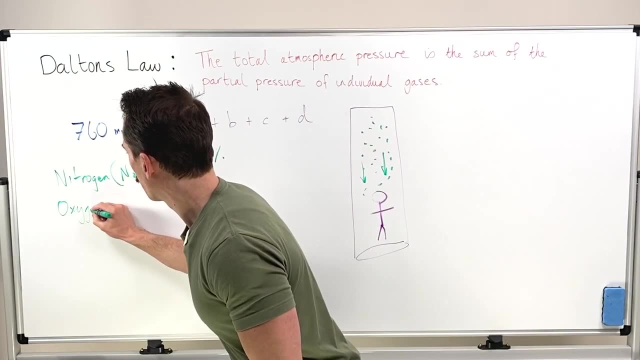 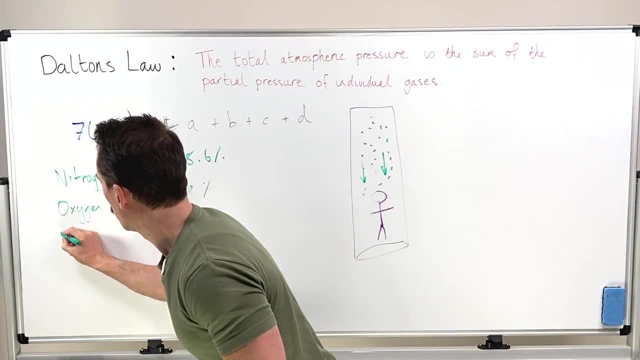 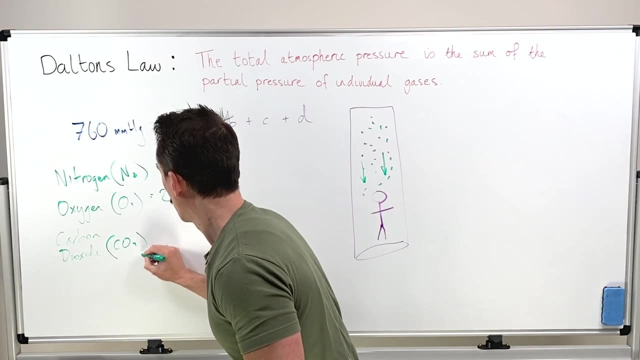 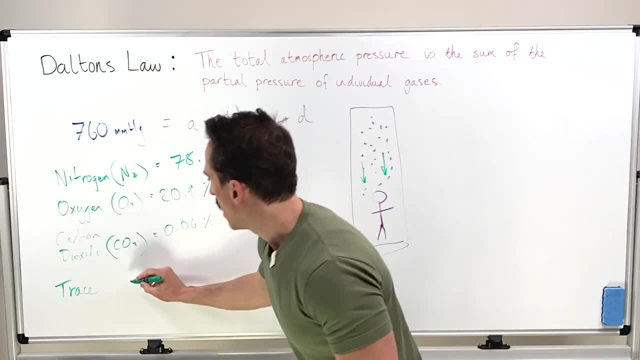 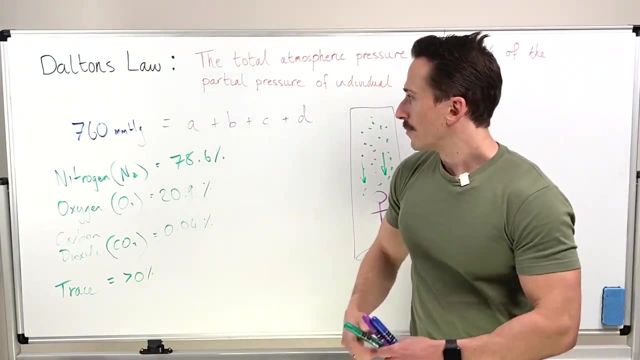 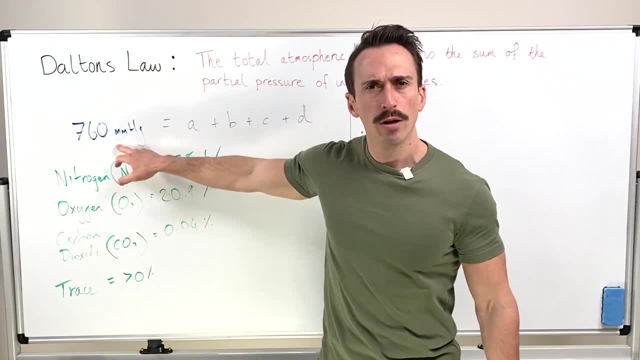 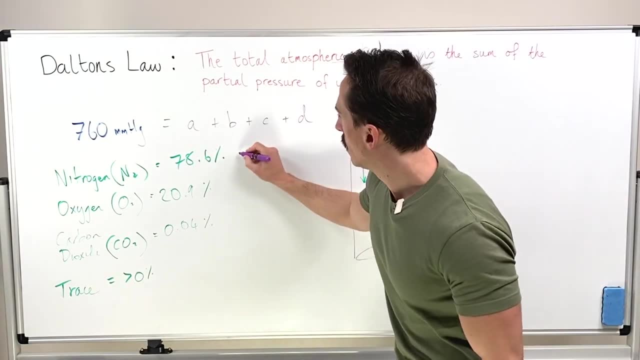 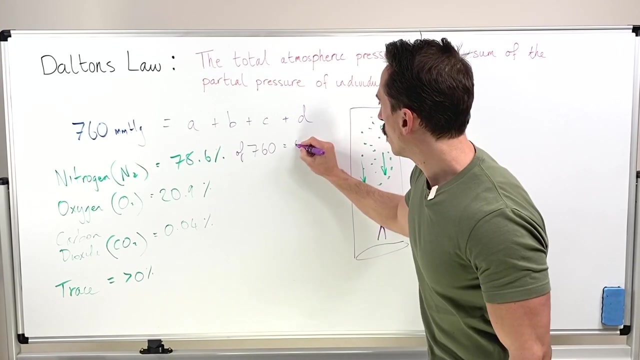 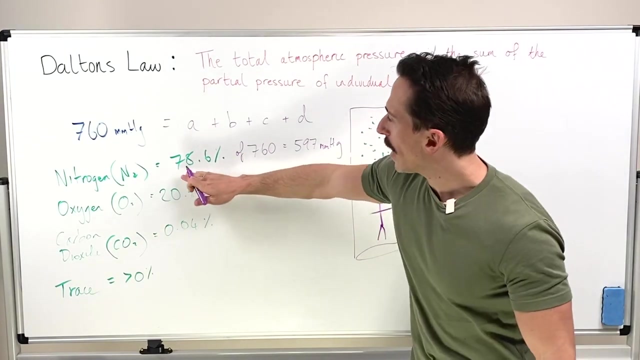 Nitrogen. Now that's a percentage and that's an actual unit of measurement, So we need to do some slight changes. 78.6% of 760 mmHg is actually equal to 597 mmHg. So you can see 78.6% of the total atmospheric pressure is 597, and that's nitrogen. 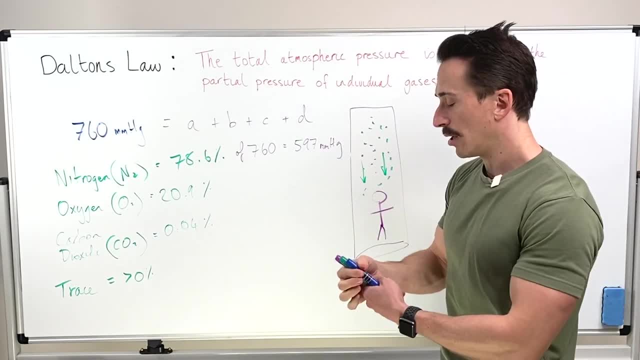 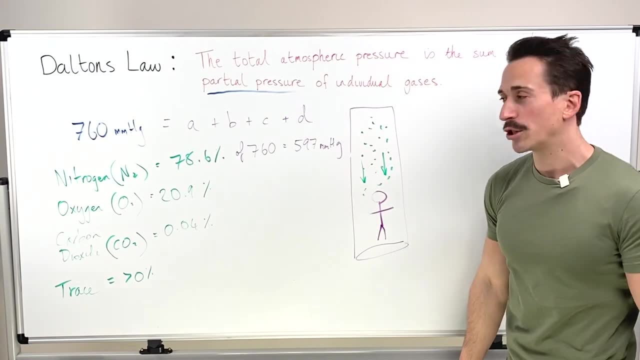 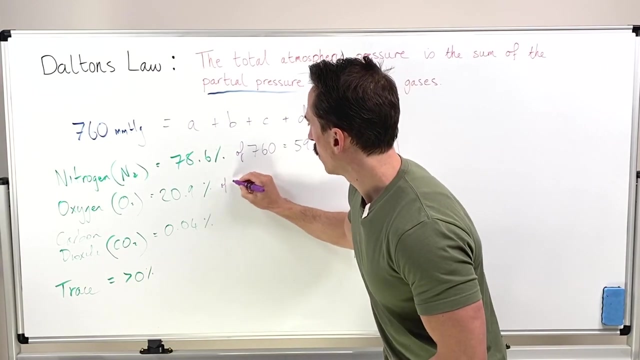 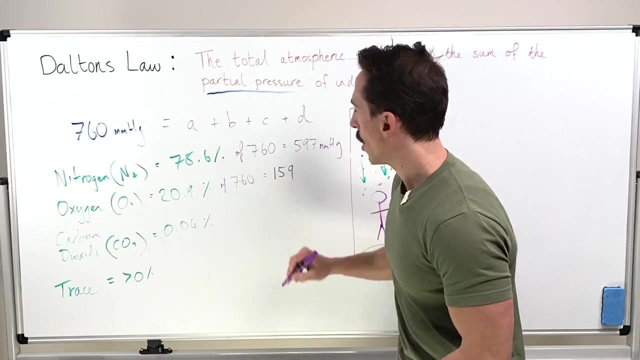 We refer to this as the partial pressure of nitrogen. The partial pressure- I think I wrote it up here, right? The partial pressure. Let's do this for the rest of them. right For oxygen, 20.9% of 760 is going to be around about 159 mmHg. 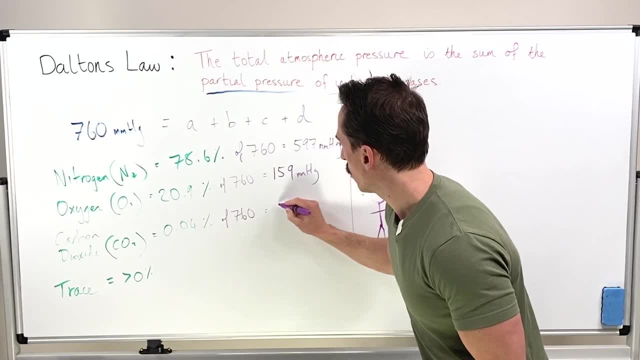 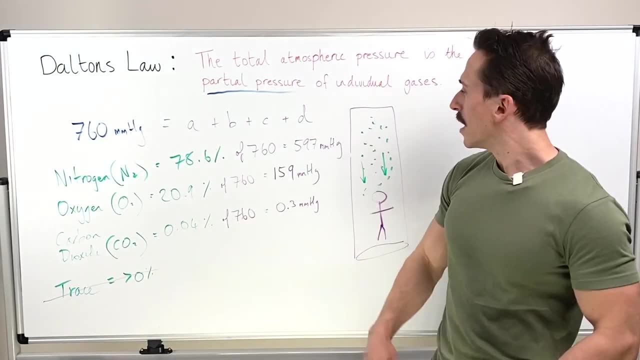 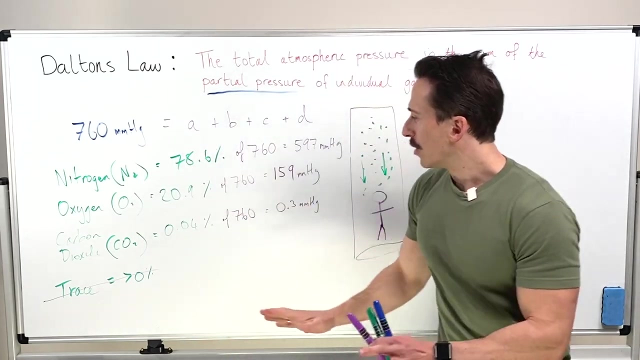 And for carbon dioxide it's going to be around about 0.3 mmHg. Let's not worry about the trace gases. So if we add those together they should be around about 760 mmHg. Now again, what we've just calculated is the partial pressure of each of those gases within. 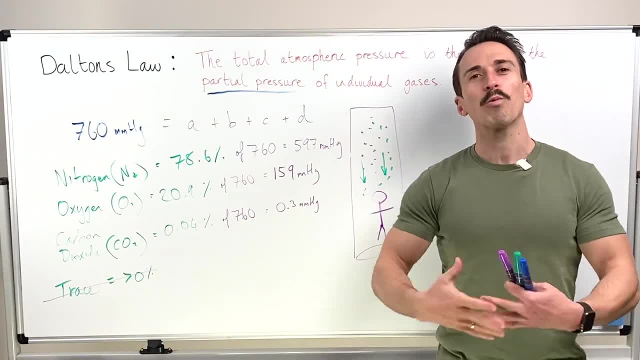 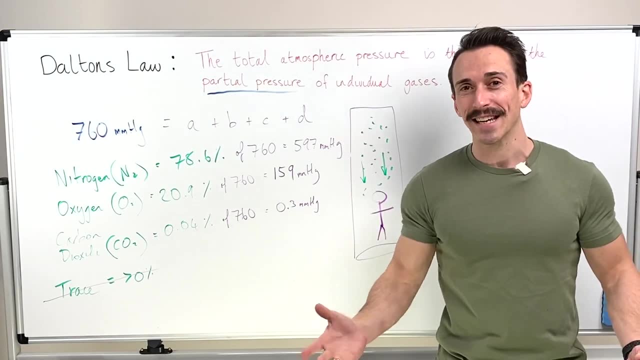 the total atmospheric pressure. You might be thinking: who cares? What relevance does this have when it comes to the physiology of breathing, Whether that be diving or aviation, or just at sea level? So let's take a look. Let's go back to this column of air. 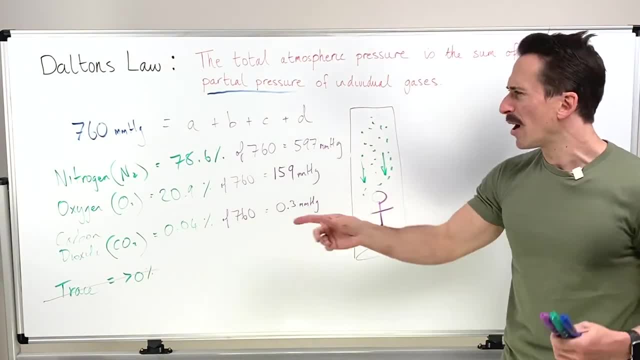 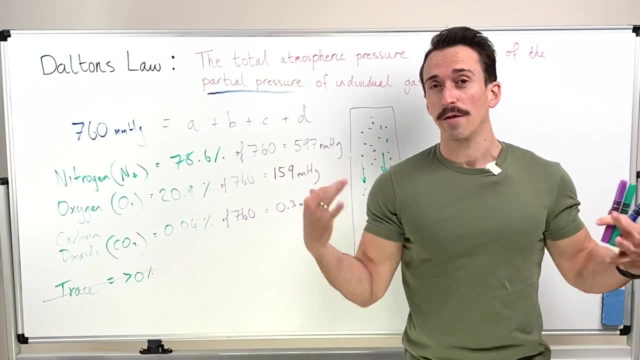 This column of air that's sitting on top of us has that pressure. You might ask: well, if it's 760 mmHg, how come I'm not feeling this pressure? It's because we're born into it, So of course we don't feel that pressure around us. 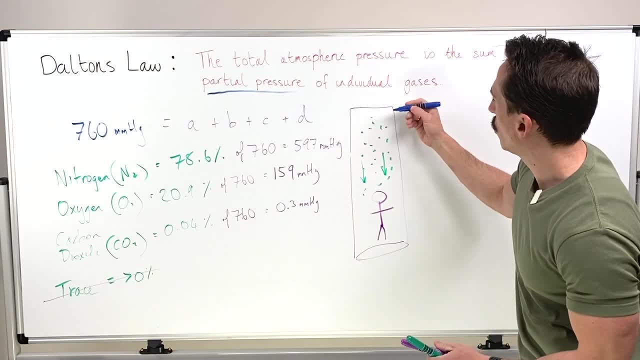 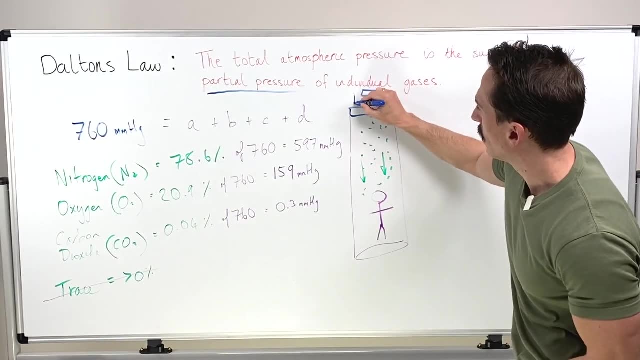 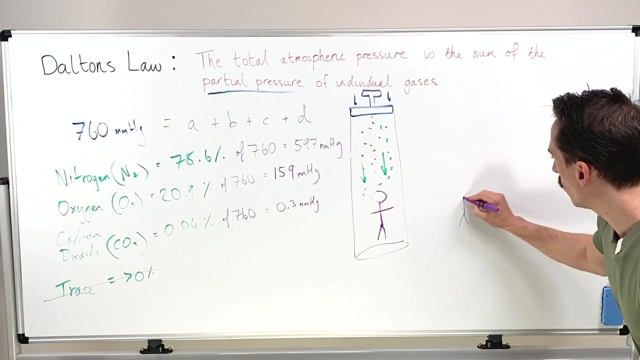 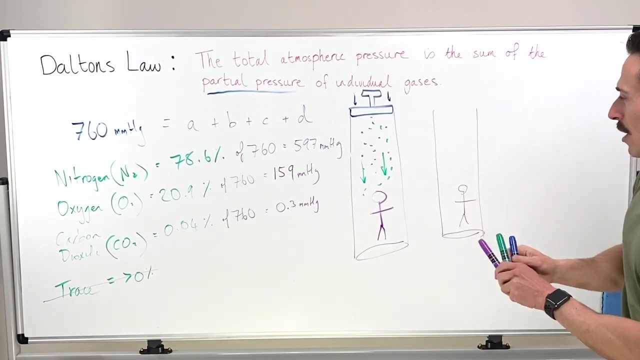 But let's just say, this column of air was attached to a syringe, barrel and plunger and we decided to push down On top, On top On that plunger. So let's just draw it up here: In this scenario we're in that tube, that column of air, but now we've pushed the same. 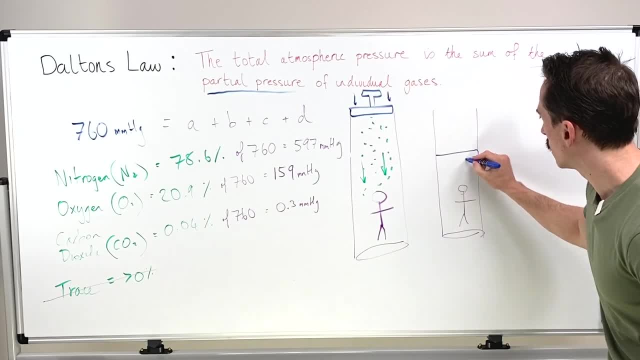 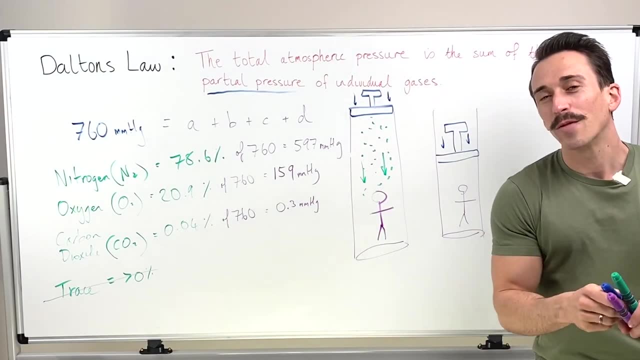 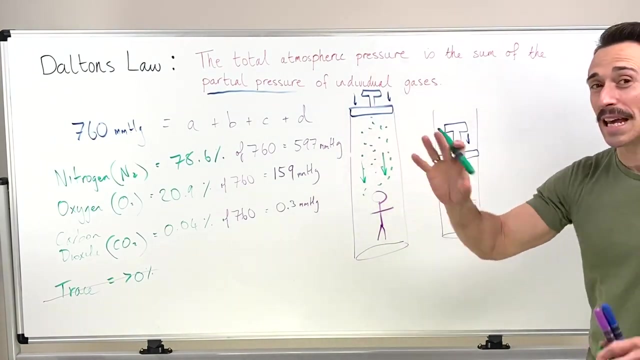 amount of gas down into less space by pushing down. Now what we've effectively done is we've increased the atmospheric pressure because of something called Boyle's Law. I've done a video on Boyle's Law, If you. there's an inverse relationship between the volume of a container and the pressure. 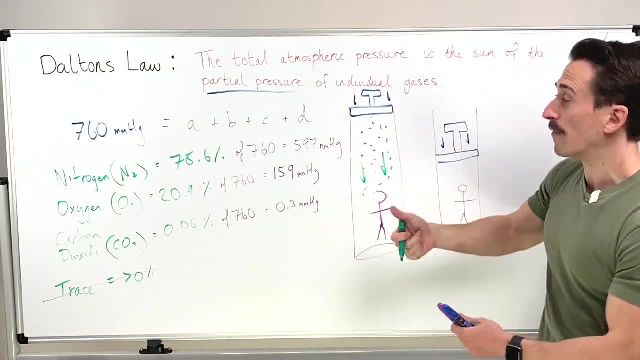 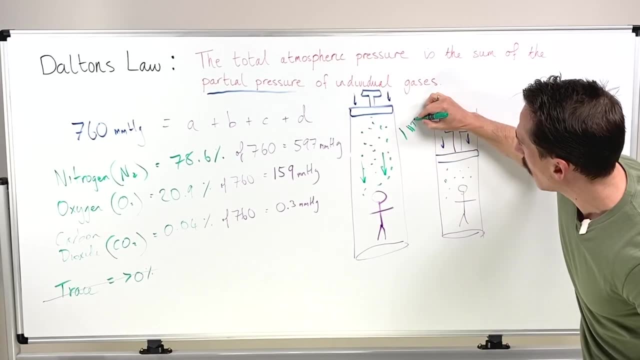 of the container. So if I decrease the volume, I've increased the pressure, and that's what's happening here. I've just decreased the volume and I've increased the pressure Instead of going from. so this is one atmosphere. I've now made it two atmospheres.